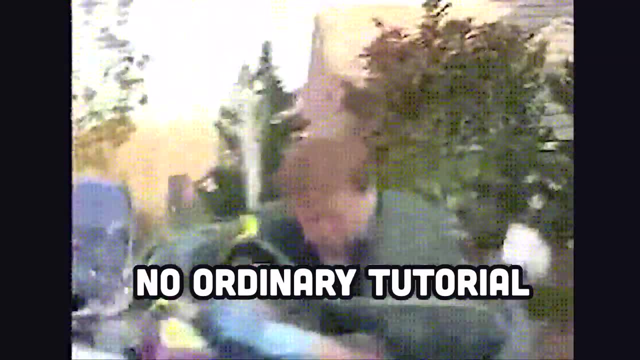 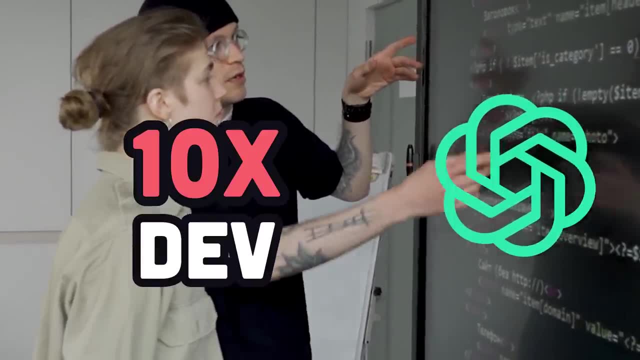 just one of millions on the internet, But it's no ordinary tutorial. It's the first tutorial to leverage the full power of AI to write code like a 10x developer, even if you've never written a single line of code in your life. What's crazy, though, is that this tutorial can be applied to 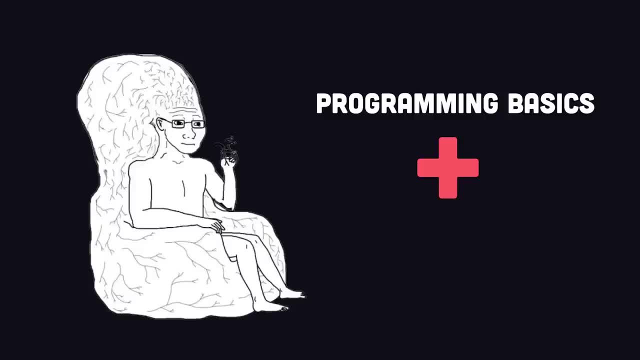 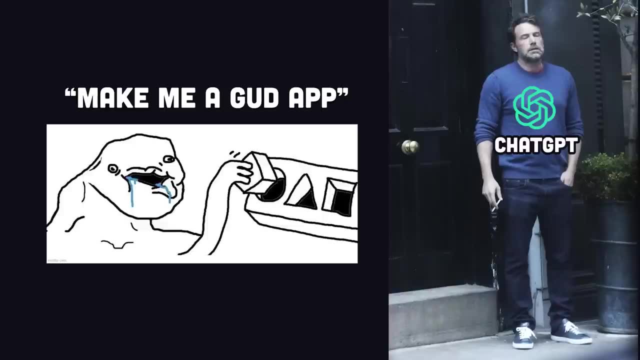 any language or framework. Once you know some basic programming principles and how to prompt like a pro, you can build almost anything in your imagination. But it's not as simple as just asking ChatGPT to build you a React app. You will need some domain knowledge and understand how to. 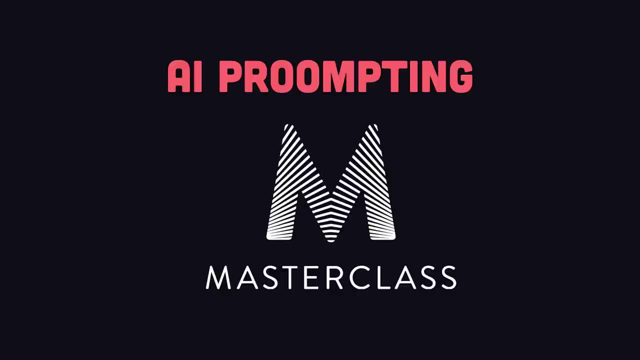 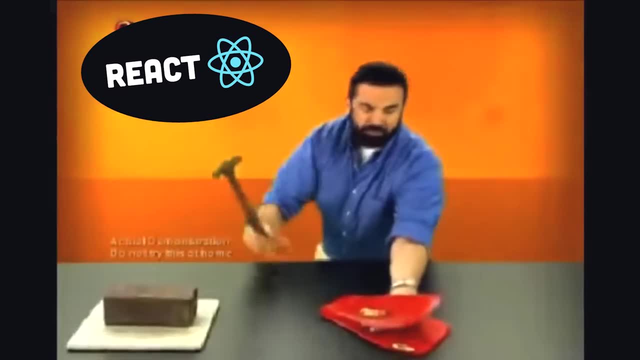 execute and validate the code that the AI spits out. Let's go ahead and get started with your AI prompting masterclass. I'm assuming you know nothing about React other than it's a library for building UIs. I could sit here and teach you about React and ask you to buy my $500 React course. 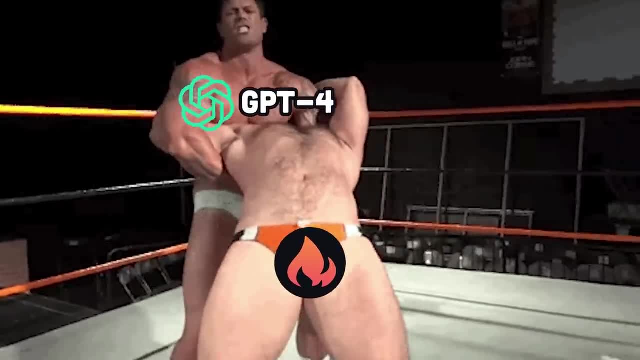 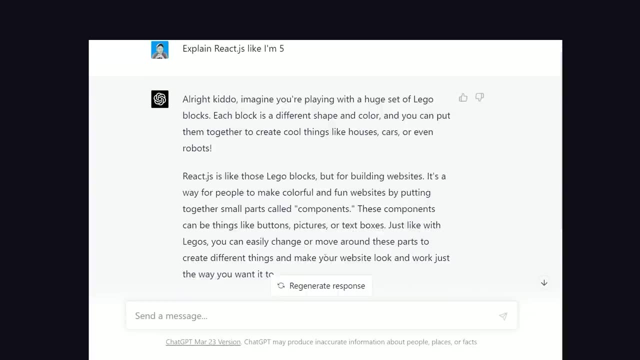 but the truth is that GPT-4 can teach you better than I can. I hate to admit it, but it's true. If you want to learn something you know absolutely nothing about, go ahead and prompt it to explain it like you're five. In this case, it'll explain how ReactJS components are like Lego bricks. 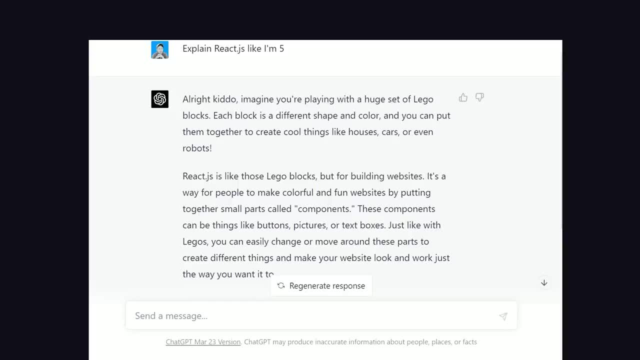 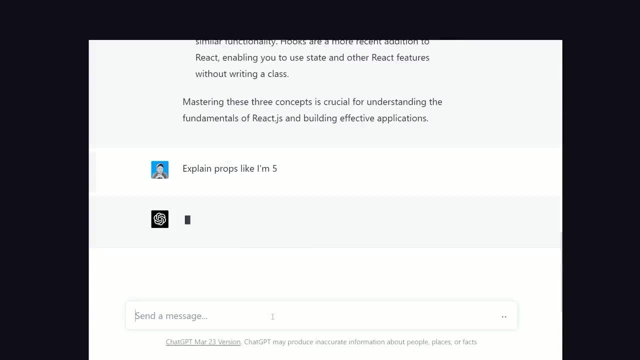 but for building websites, which is the perfect metaphor. From there, I ask it for the most important concepts that I should know. It then explains components, state and props and hooks. If there's anything you don't understand here, you can then prompt it to. 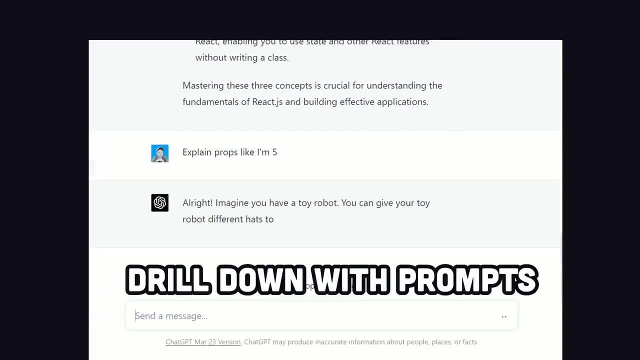 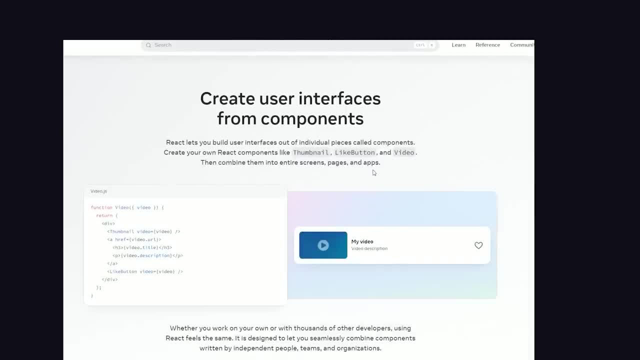 explain that one thing in more detail, or explain that to you like you're five. One problem, though, is that LLMs tend to hallucinate aka make stuff up, So, as of today, it's not really a replacement for the ReactJS documentation, which is excellent, by the way. However, ChatGPT has a browser plugin. 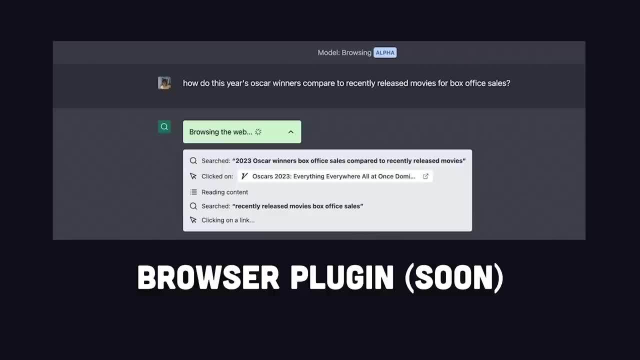 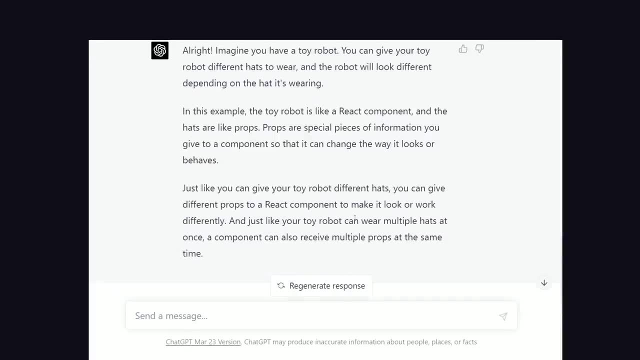 that's on a waitlist right now, which will eventually solve that hallucination problem. So the ReactJS docs are like the Bible and ChatGPT is like a priest, who makes all the money but sometimes invents his own ideas. Now, once you have a general idea about the 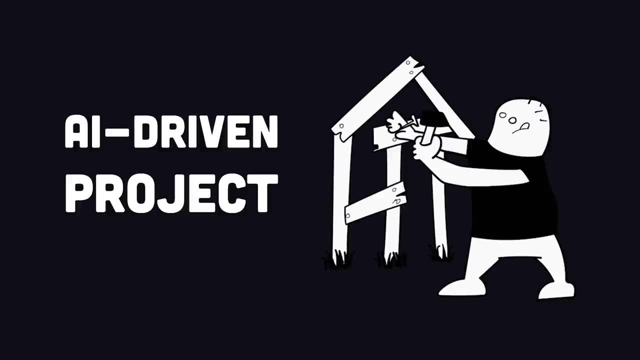 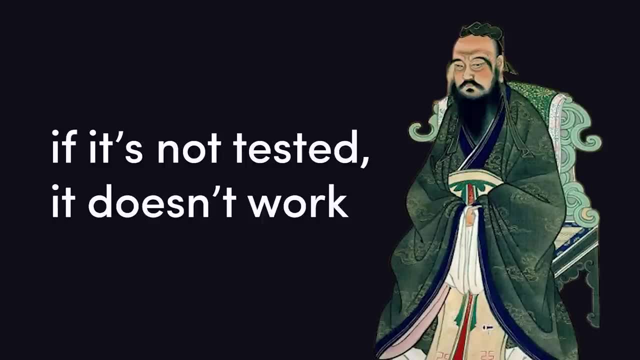 language or framework that you're trying to build with. the next step is to set up a project that allows you to inject AI code in a safe and effective way. There's an old programming proverb that says if code is not tested, it doesn't work, And that's especially true when 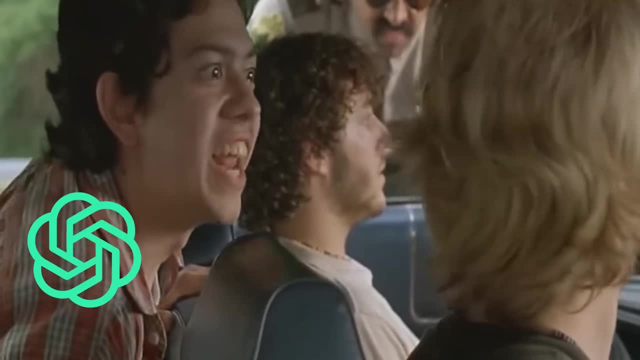 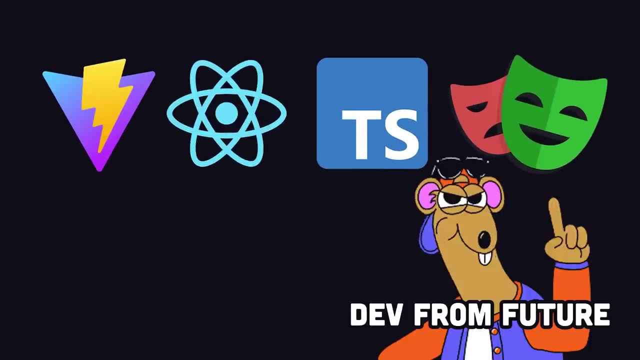 working with an AI that acts like it's tripping balls. I'm freaking out, man. As someone who's done a lot of React development, I'm just going to do it the old fashioned way and set the project up the way I want it- manually. But doing things like this is very 2022.. Like yesterday on Twitter. 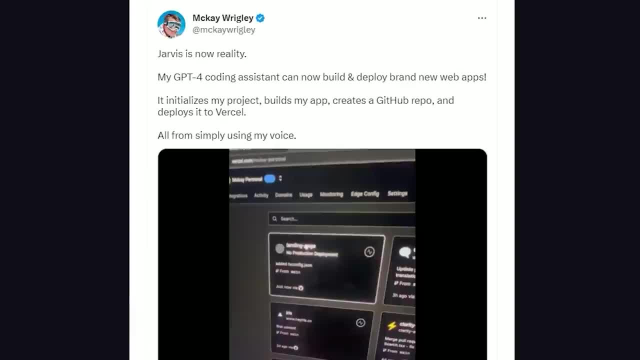 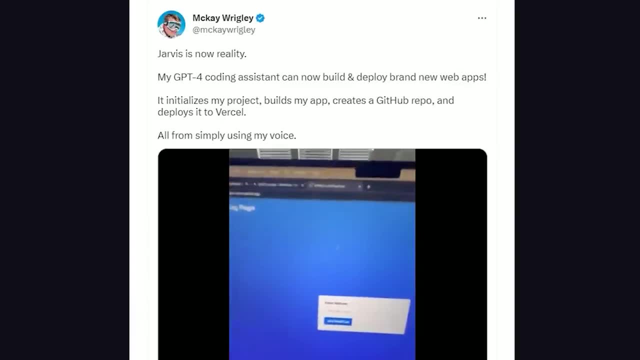 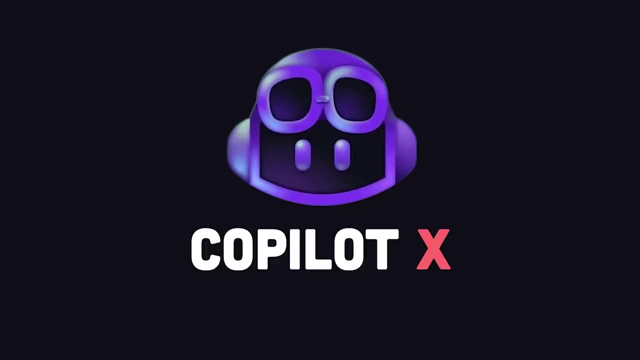 I saw this guy set up and build a project entirely from voice commands and then deploy it to Vercel, Which means it did in fact deploy Dude. it did it. It nailed the background. No way I'm using VS Code from Microsoft as my editor. It's not available today, but GitHub Copilot X. 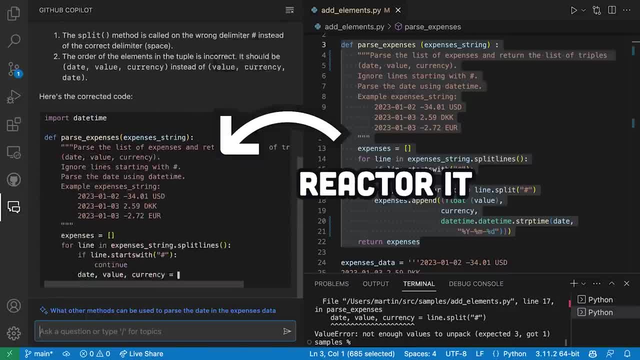 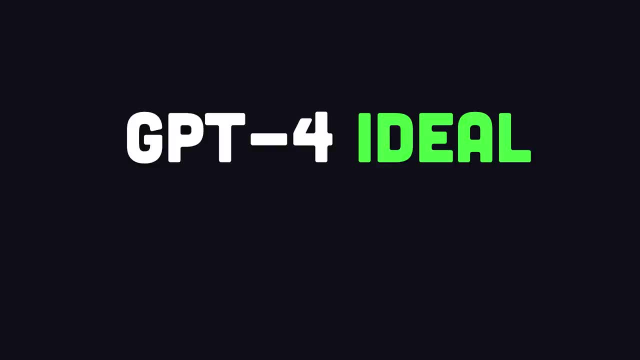 is coming, A plugin for VS Code that brings ChatGPT directly into your editor. Make sure you're subscribed for the latest updates on that tool. The only other tool you'll need is ChatGPT, ideally with GPT-4,, which is currently paid, but 3.5 will work as well. Here I have VS Code open. 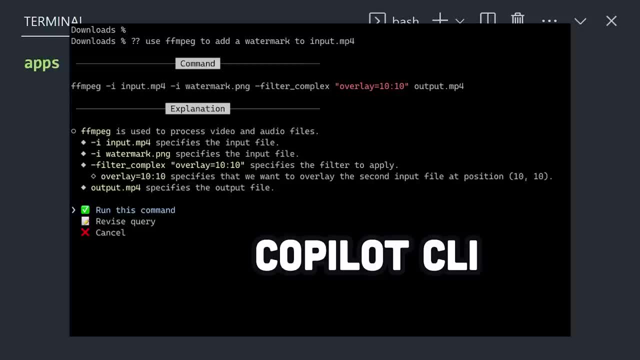 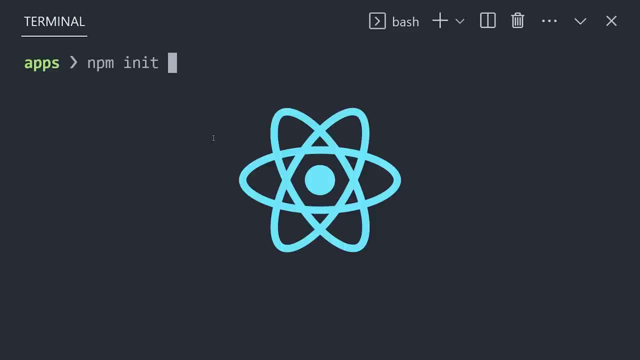 to my terminal with Nodejs installed. In the future we'll have tools like GitHub, Copilot, CLI that can find and explain commands for us, But for now I'm just going to initialize a new React project with VEETjs. We'll go ahead and use TypeScript, because I have some TypeScript tricks. 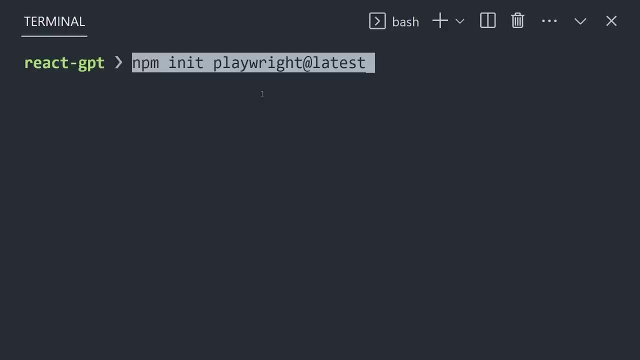 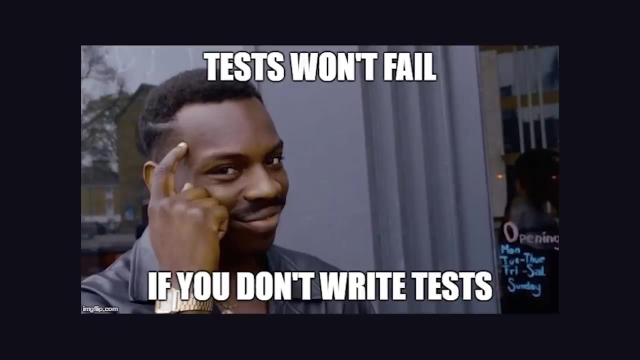 to show you And then, once inside that project, we'll go ahead and install another tool called PlayWrite for end-to-end testing in the browser. When developing an app, testing is technically not required, but it's extremely important when working with AI, because we need to validate that. 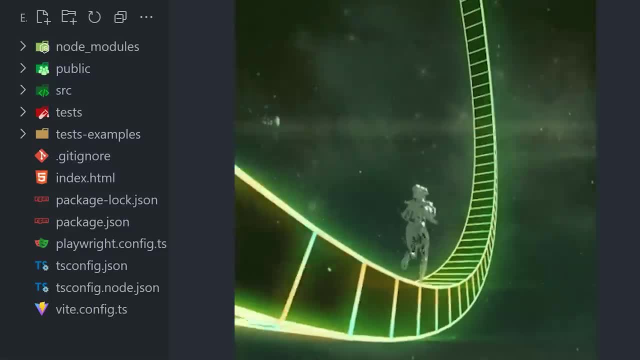 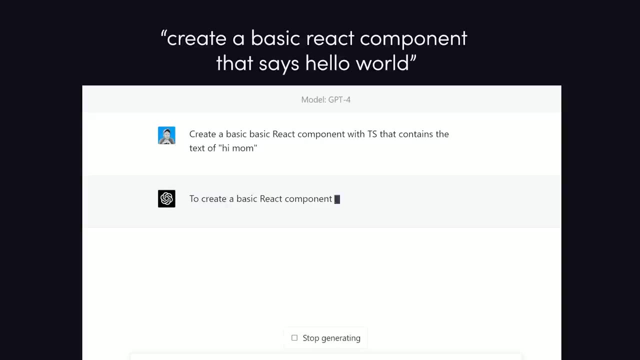 it does what it's supposed to. The good news, though, is that AI can write its own test, as we'll see shortly Now. the main component in the source directory is in the apptsx file. Let's go ahead and prompt ChatGPT to replace it with a more basic Hello World. GPT-4 is kind of 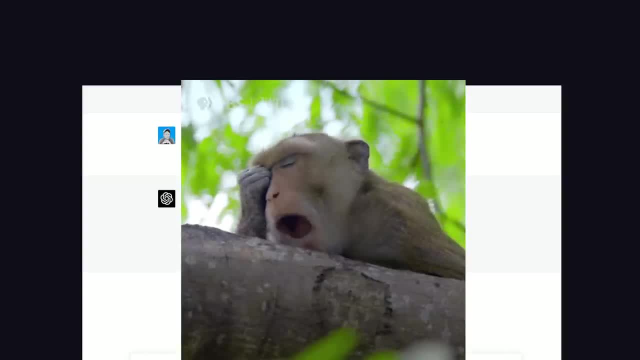 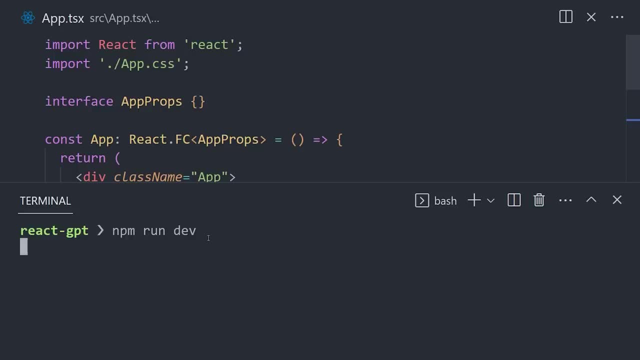 slow and can often be overly verbose. So one thing you can do is just say code only to shorten the response. That looks pretty good. Let's copy and paste it into our project. Now go to the terminal and run npm, run dev, and you should get this Hello World component. But that's a little too simple. 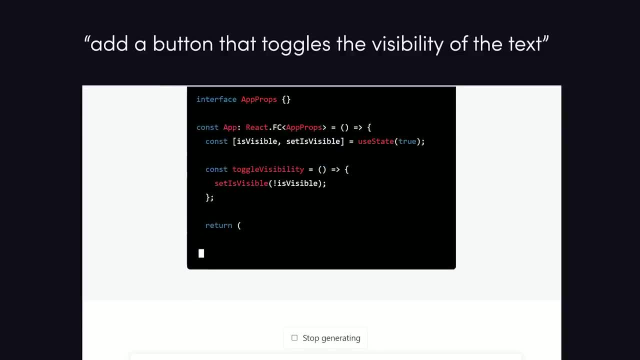 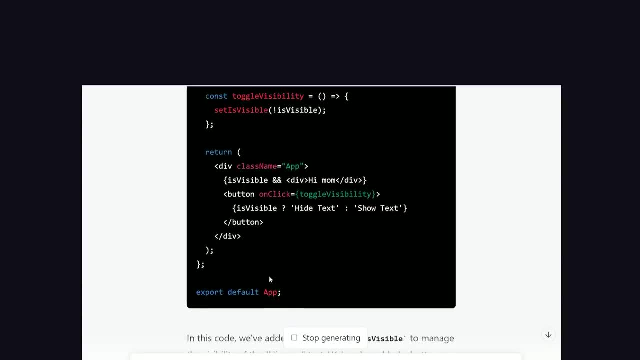 Let's go back to ChatGPT and now have it modify this code with a button that will toggle the visibility of the Hello World text. When doing that, it explains how we'll need to use React State to manage the visibility. Paste the updated code into your project, save it, and now you have. 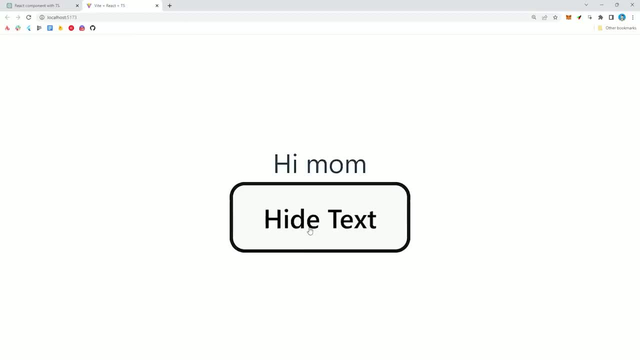 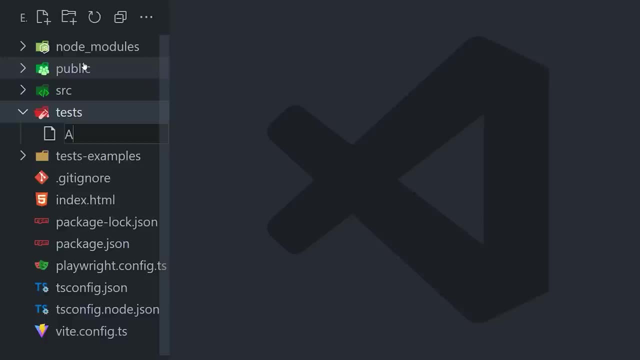 a working interactive React app. That's pretty cool, but we want to make sure that the AI doesn't accidentally break this code in the future, so let's ask it to write a test with PlayWrite Once again, copy the code, then go into the test directory and create a new file called apptestts. 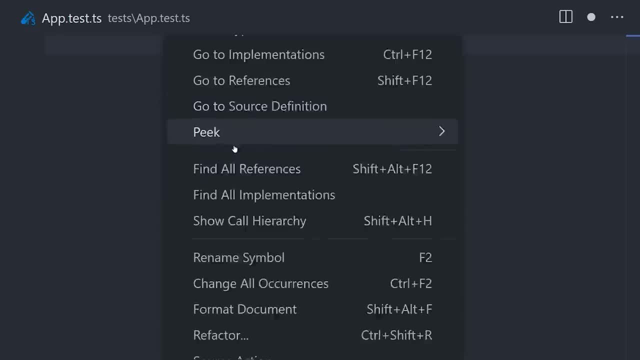 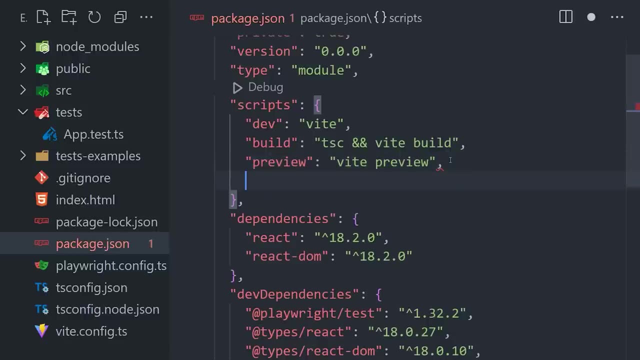 Here's a pro tip. as a prompting engineer, You can use Ctrl-V on your keyboard instead of doing right-click-paste, to maximize your speed Now. from there, you'll see that you'll be able to run a test with PlayWrite. From there, we need to go into the packagejson file and set up a. 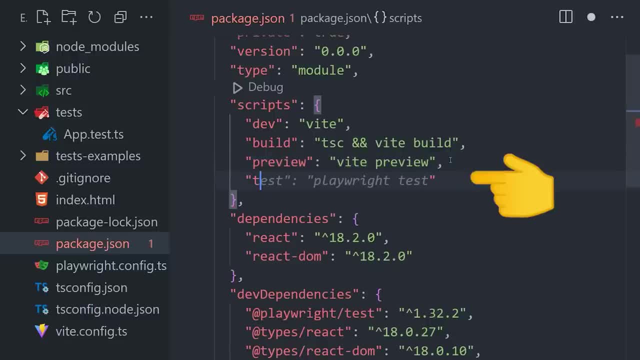 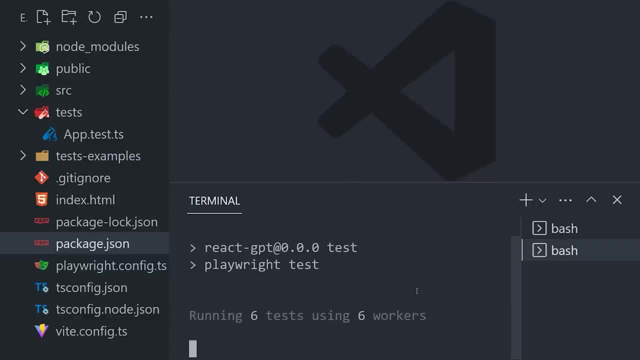 testing script. If you already have Copilot installed, you can just type test and it should automatically detect PlayWrite and create the script for you, which is just PlayWrite test. From there we can open the terminal, run npm, run test and PlayWrite will test this code on. 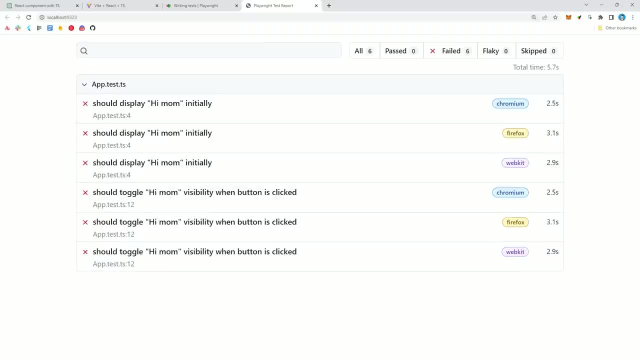 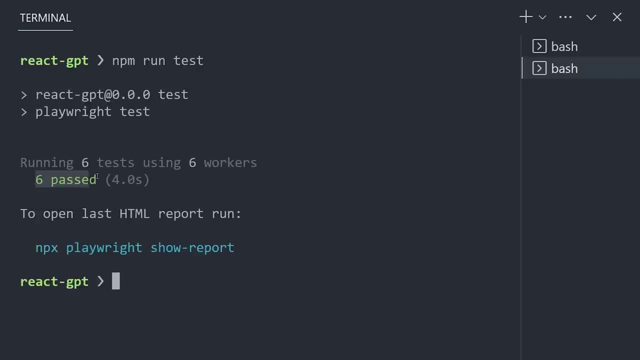 multiple browsers in parallel. As you can see, it fails because we don't have the right localhost port setup. so let's go ahead and modify that in our testing code and run it again. This time it passes. In the future, GitHub Copilot will know the full context of your project and won't make 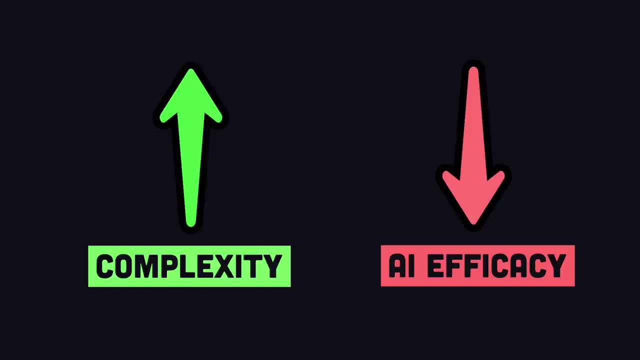 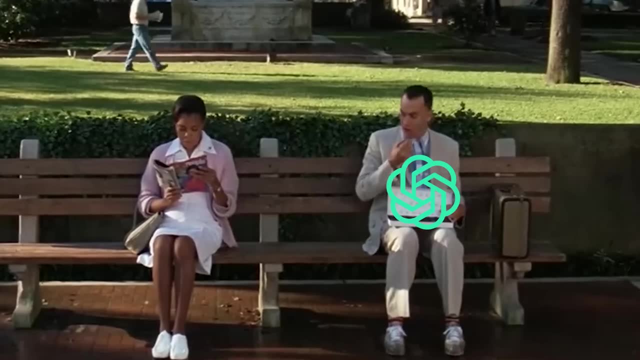 any changes. This is cool and all, but what you'll find. as your app grows more and more complex, it becomes harder and harder to prompt the AI effectively. It's non-deterministic, which means you can get different results from the same prompt. You never know what you're gonna get. 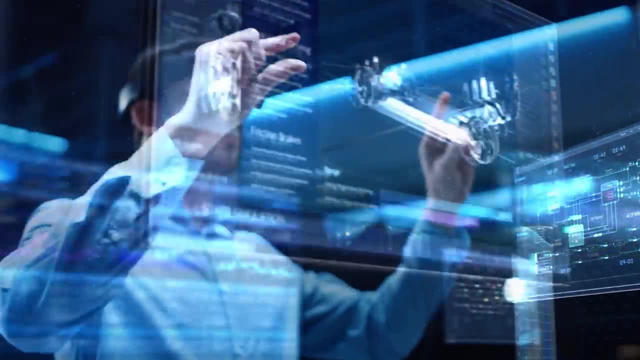 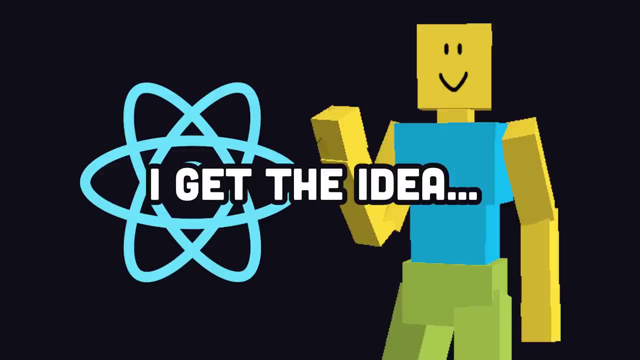 And that's complete madness for a programmer. But now here's where things get really mind-blowing, and we'll give you a glimpse into the future of programming. At this point you have the general idea of how React works, but you may not know JavaScript very well or haven't memorized all. 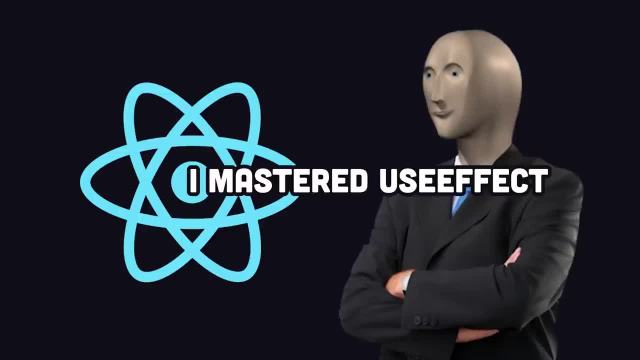 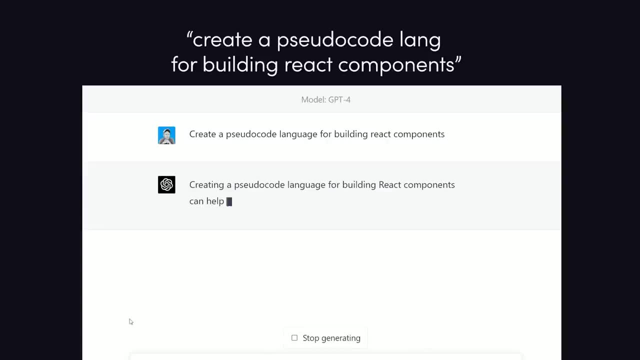 the little quirks in the framework. Or maybe you're a React expert and just don't want to go through the tedious process of writing perfectly structured code. So what we can do next is have ChatGPT come up with a pseudocode language for React. What this? 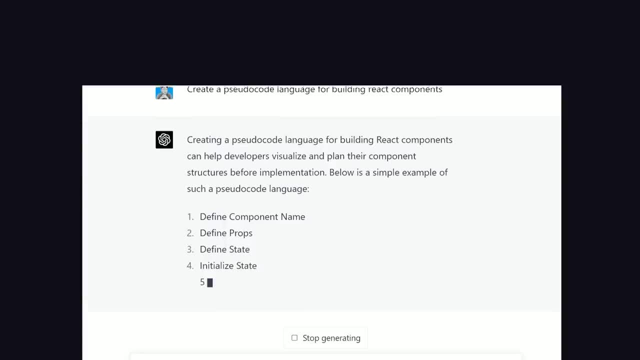 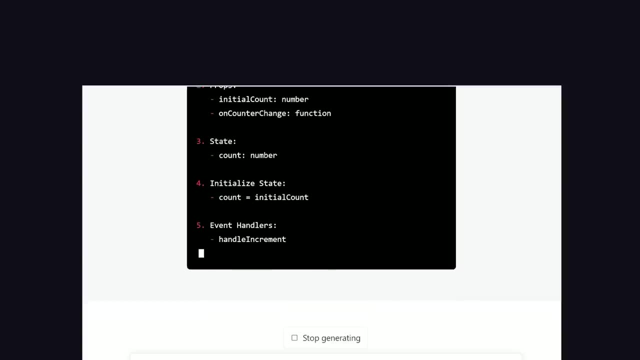 will do is allow us to agree on some general guidelines to represent the structure of a React component. As you can see here, it looks kind of like YAML and allows us to define state and then the rendering function or JSX, And if we don't like the way it looks, we can tell it to come. 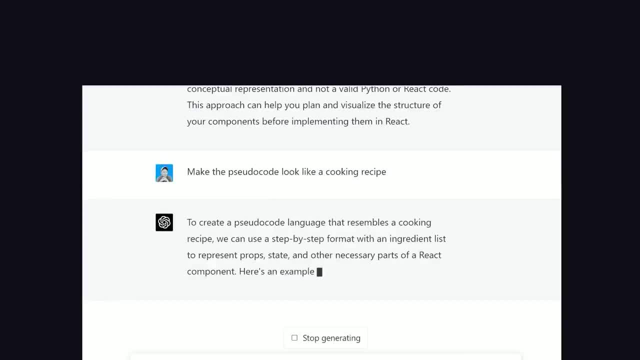 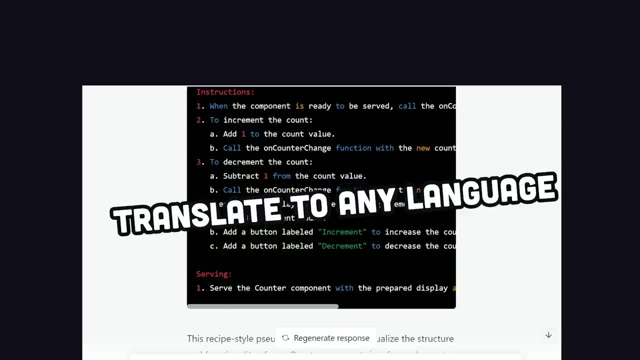 up with a different idea, like: maybe make it look more like Python. Actually, no, let's make it look like a cooking recipe, which is surprisingly a very intuitive way to represent a React component. And, as an added benefit, you could write this in any human language and have it translate your. 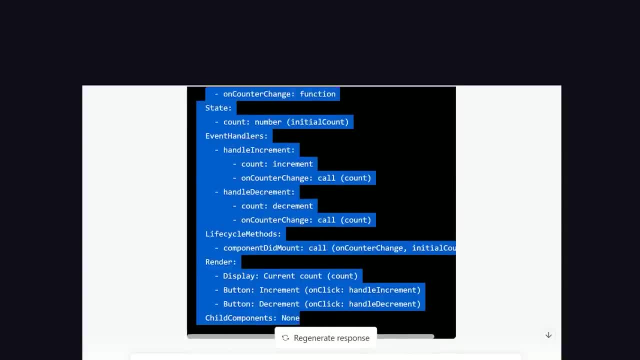 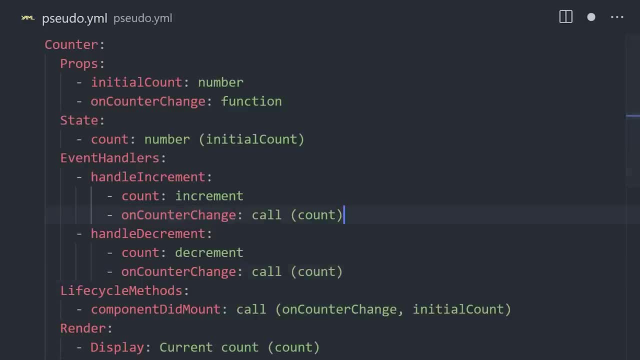 code back to English, But from a practical standpoint, I think you want something that kind of looks like YAML. Overall it's way more concise and doesn't require us to use precise syntax, but at the same time it will give us relatively consistent results And we can make. 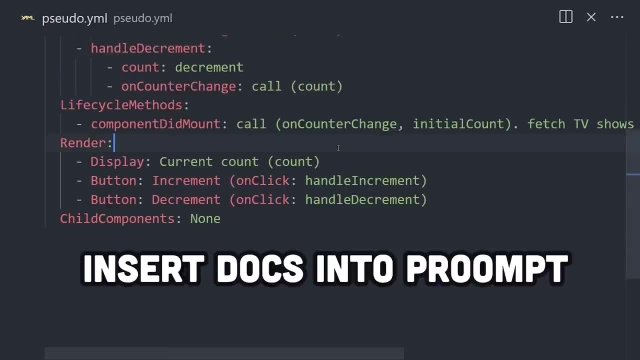 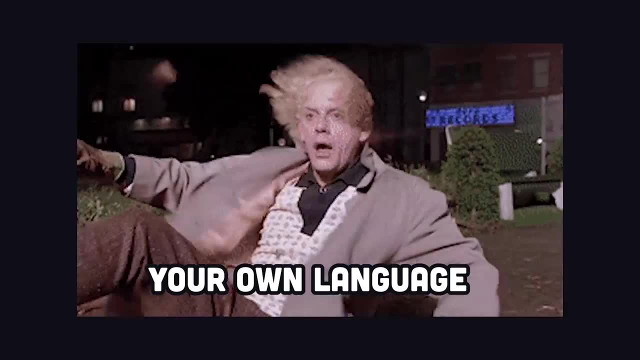 it even better by including relevant documentation or a style guide to force it to write code in a style that fits our project. because GPT-4 can now handle up to 25,000 tokens, The end result is your own custom AI pseudocode language, As you can see here. 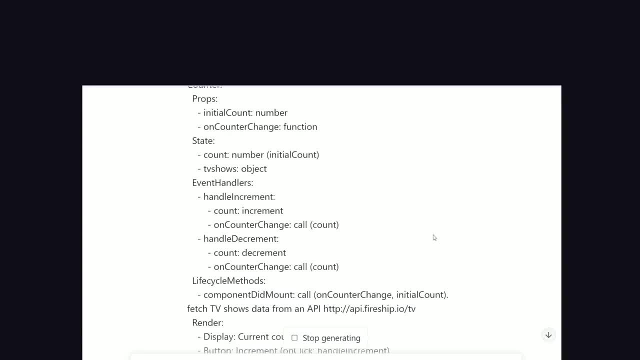 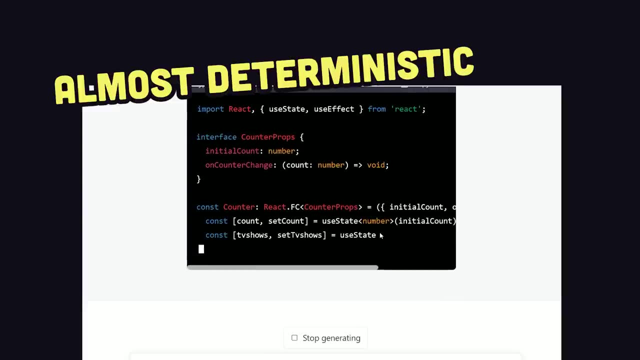 I wrote out a relatively complex component in this language and it generates perfect React code as a whole, But, most importantly, it generates the same code every time, most of the time, maybe 80% of the time. This is pretty mind-blowing, because now any developer can have their own. 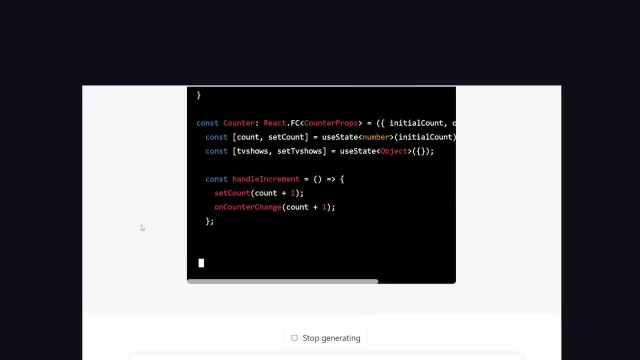 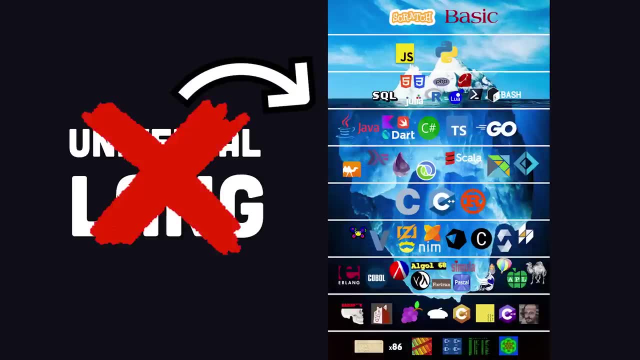 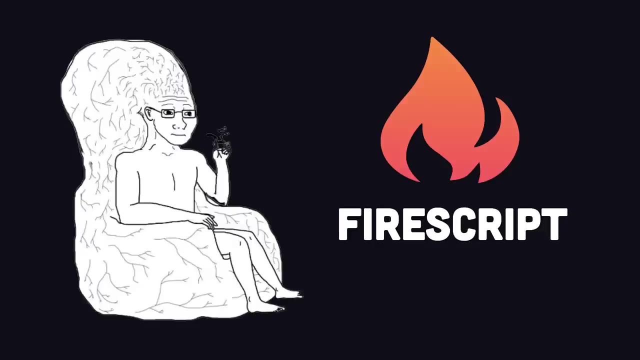 custom tailored pseudocode language that can transpile into complex code in virtually any language without understanding the underlying syntax. In a previous video, I predicted that someday there will be a universal AI language, but maybe I was wrong. Maybe every developer gets to build their own AI language, custom tailored to optimize their own productivity. 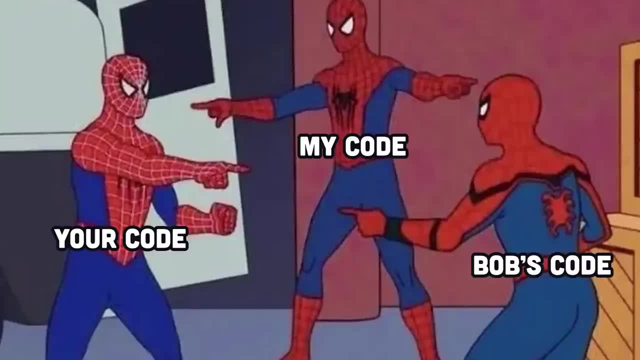 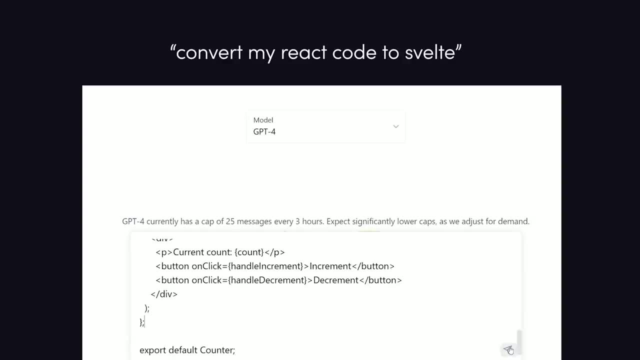 Sounds like chaos on a team, but AI can also translate your pseudocode into my pseudocode and my pseudocode into your pseudocode. In fact, one thing we could do right now is take the generated React code and convert it into a superior framework like Svelte or Solid. 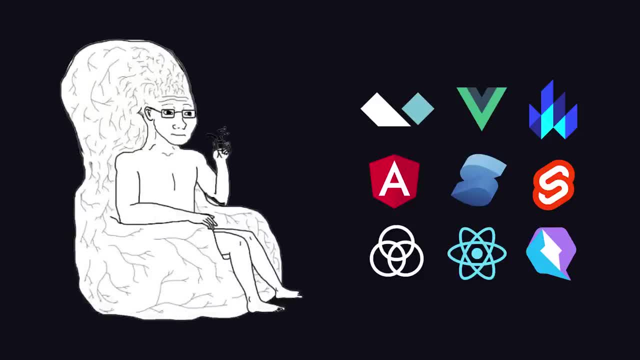 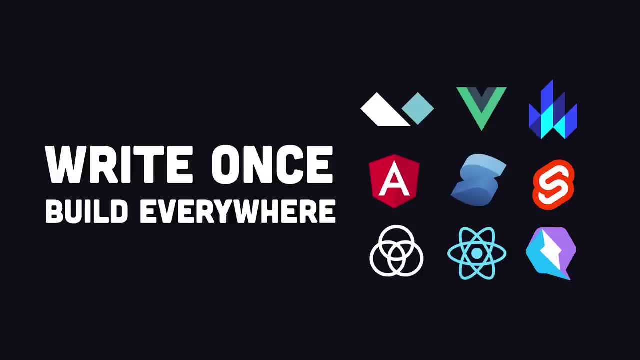 There's a million different JavaScript frameworks out there, but now we can use them without learning them. In fact, we could use our pseudocode to build the same app and multiple frameworks at the same time, then benchmark their performance and just choose whichever one performs the best. 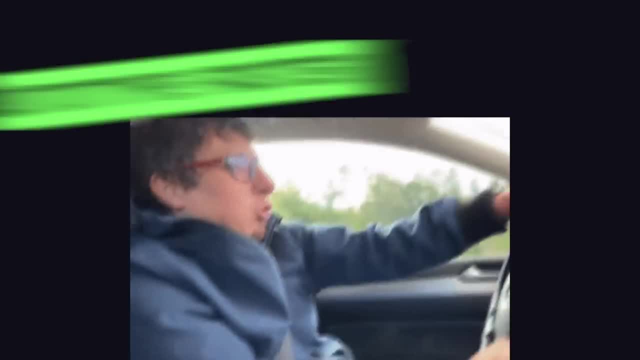 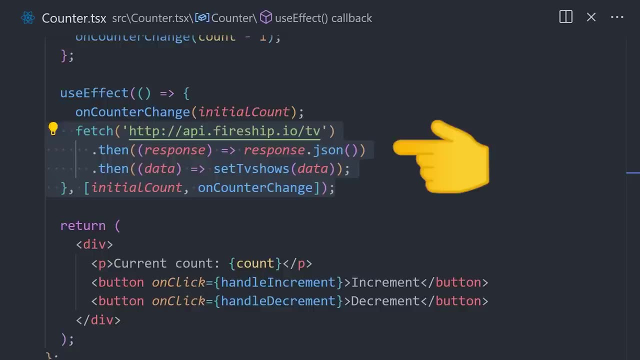 That's more of a futuristic idea, but currently the main value of pseudocode is just getting things done faster without allowing the AI to become too magical, Like in this example. you can see we're making an API call, but currently we don't have any kind of interface for the response. 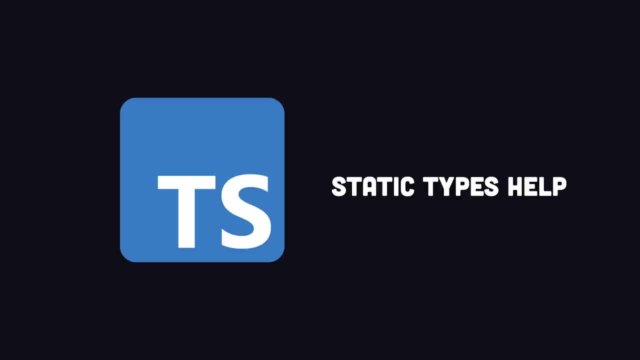 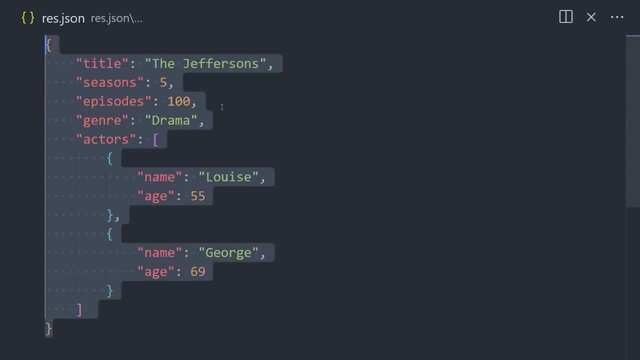 Generally speaking, GPT-4 will provide better results when you have statically typed code like TypeScript, or even just type hints in a language like Python. In this case, I have a JSON object and what I'll do is paste that into ChatGPT to turn it into a TypeScript interface. 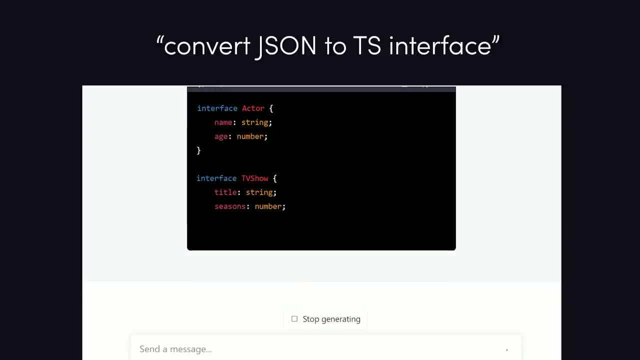 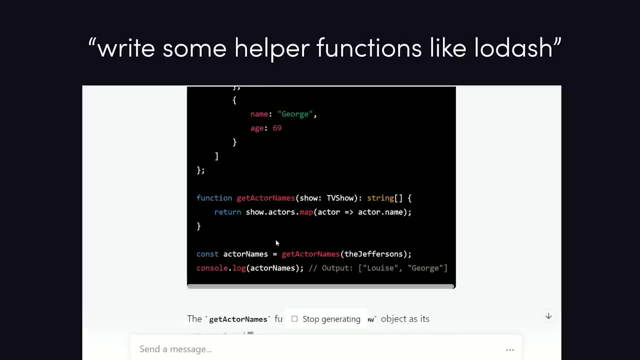 It's able to detect the two different entities of TV shows and actors, and now we can use it in our code. Now that ChatGPT has this interface, we can also tell it to generate any kind of helper functions we'll need, like if we wanted to map this object to all of the actor names. 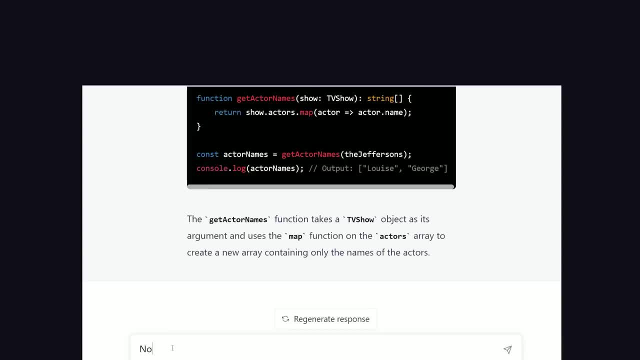 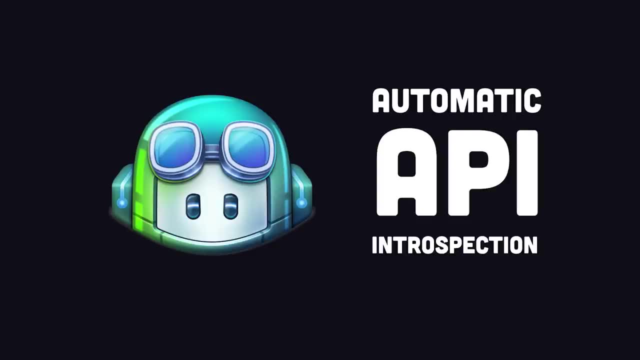 That's a pretty handy trick right now, but, once again, in the future it won't be necessary. Tools like Copilot will be able to introspect any API to provide you with automatic end-to-end type safety without any effort on your part. Now, the final thing we need to do as a 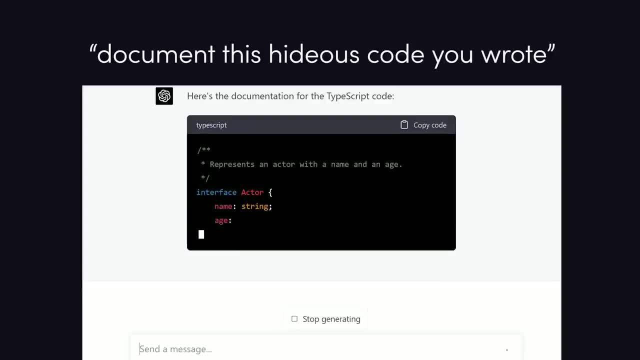 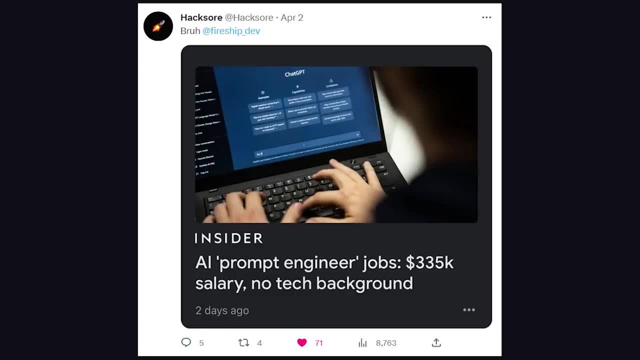 Prumpt engineer is document our code. We simply take the code we've already generated and tell ChatGPT to document it. Congratulations, you're now a 10x React Prumpt engineer. The starting salary is about $335k. This productivity boost is both exciting and scary. 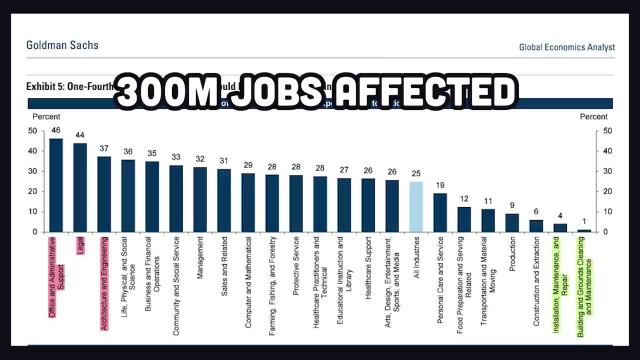 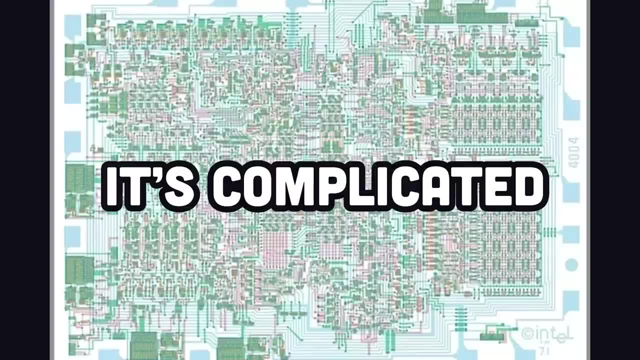 Goldman Sachs just released a report saying that 300 million jobs could be affected by AI in the near future. but there's no reason to be afraid. Software systems in real life are complex beyond belief and not even state-of-the-art AI will want to touch that code.